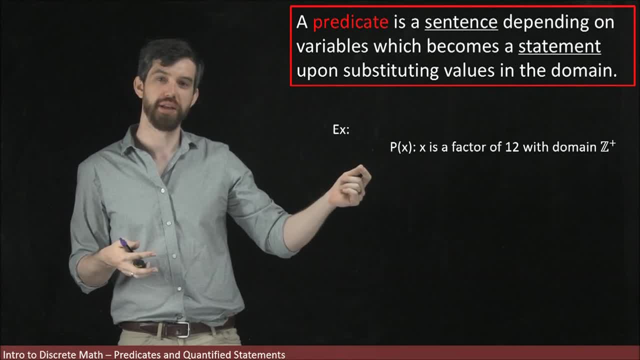 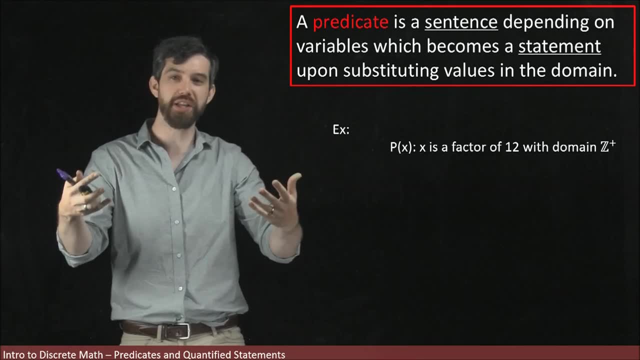 is going to be the positive integers, And the first point to note is that every predicate has to be paired with a specific domain. If I have some property that depends on x, I also need to tell you where do the x's live. 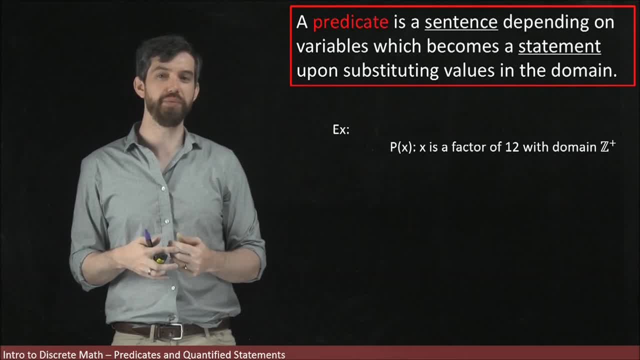 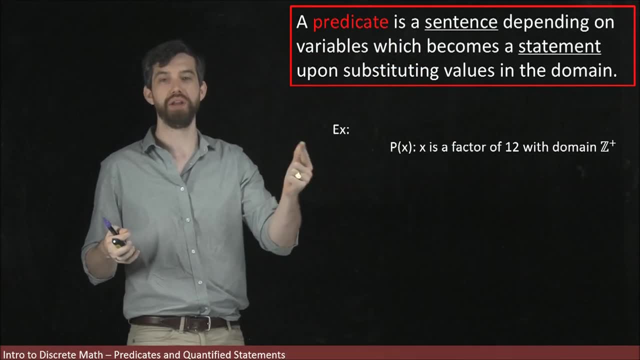 What are the allowable inputs? So, in this particular case, what I have is I've said that my domain is going to be positive integers, Numbers like 1,, 2,, 3, and so on. So now that I have this predicate, 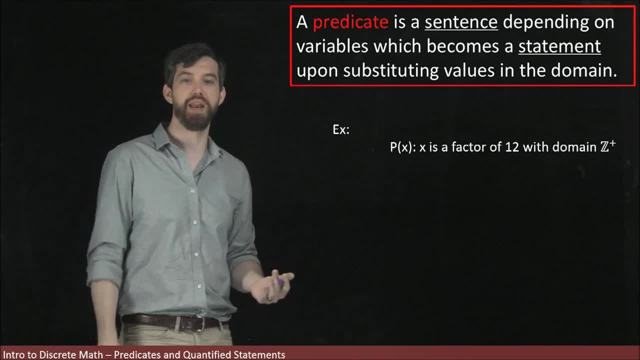 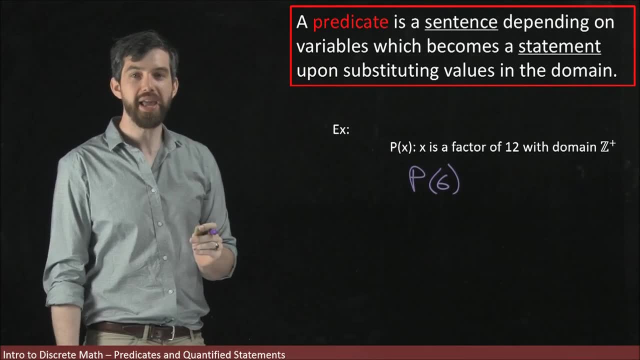 I could see whether it's true or false if I plug in a binary, If I plug in a bunch of different values. So, for example, if I take p of 6,, well, since my statement was, x is a factor of 12,. 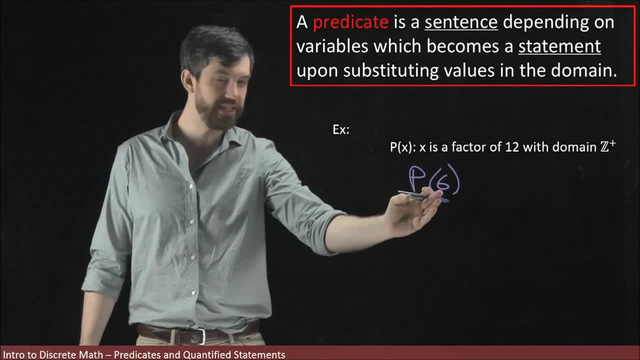 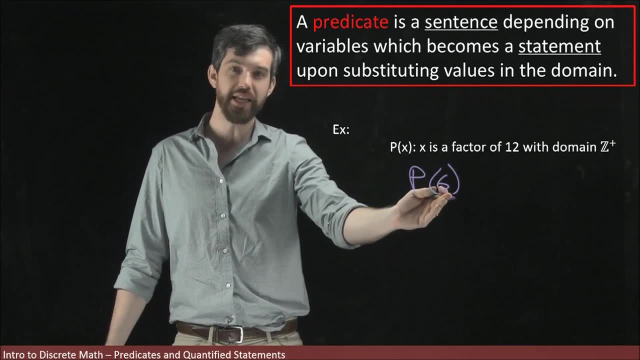 and it has to be where your x's are in the positive integers. this is it makes sense, because 6 is a positive integer, so I haven't broken any rules And 6, indeed, is a factor of 12, and so this is going to be true. 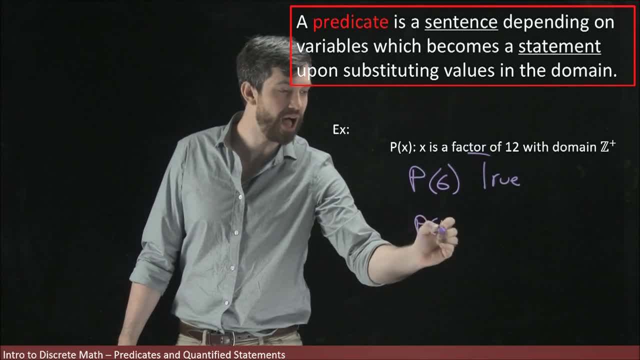 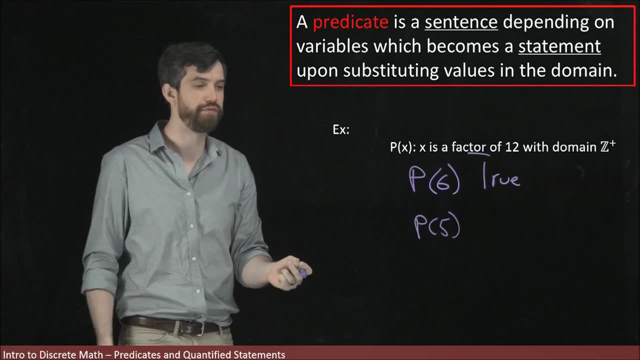 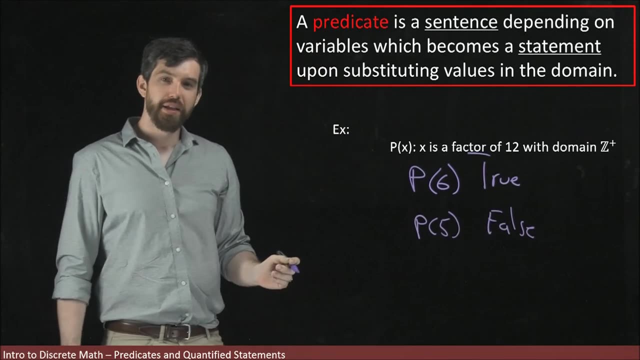 However, if I was to take something like p of 5,, well, 5 is a positive integer, but it is not a factor of 12.. So, since 5 is not a factor of 12, this is going to be false. 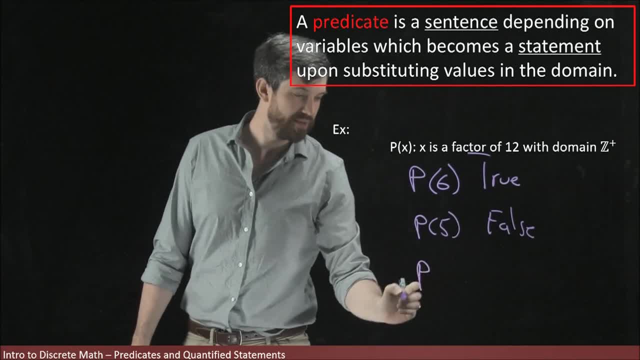 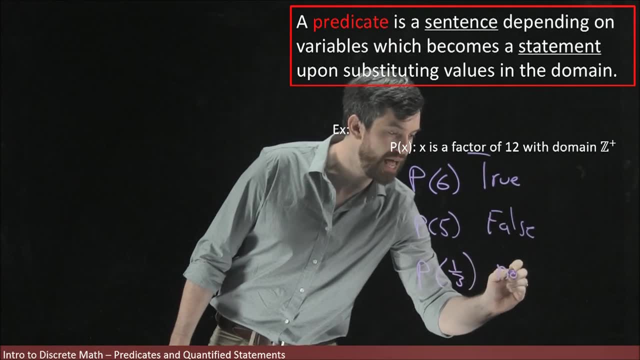 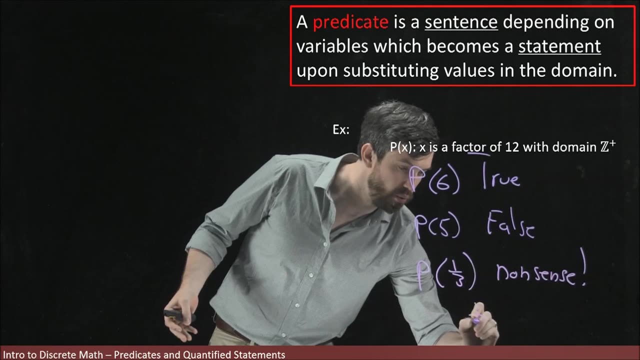 And then if I wanted to look at something like p of a third, well, this just doesn't make any sense. This is neither true nor false. It's just sort of nonsense. And the reason this is nonsense is that 1 third is not an element of the positive integers. 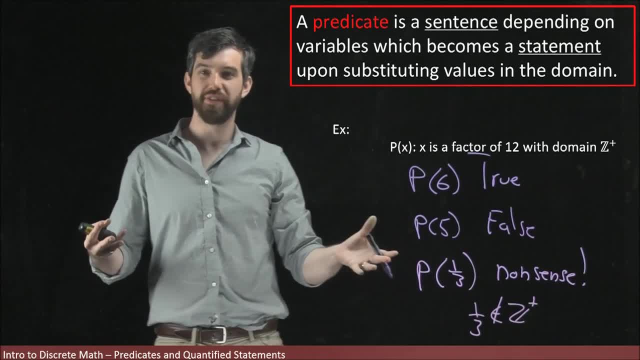 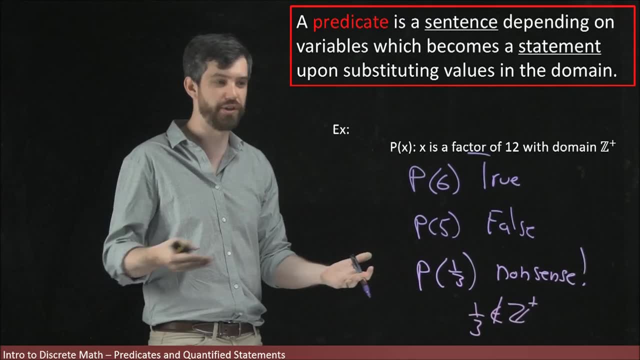 So I'm not worried about situations like this. This is sort of not a grammatically correct utterance to make, because you have this problem that the 1 third is not of the positive integers, but this particular predicate only makes sense for positive integers. 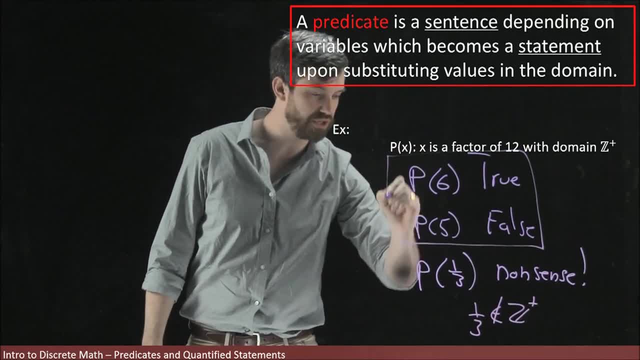 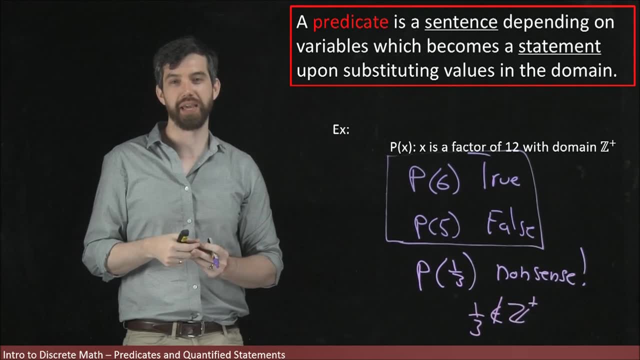 But in the two scenarios where I have plugged in positive integers, we are going to get it becoming a logical statement that's either true in the case of 6 or false in the case of 5.. If I have a predicate, I can define something called the truth set. 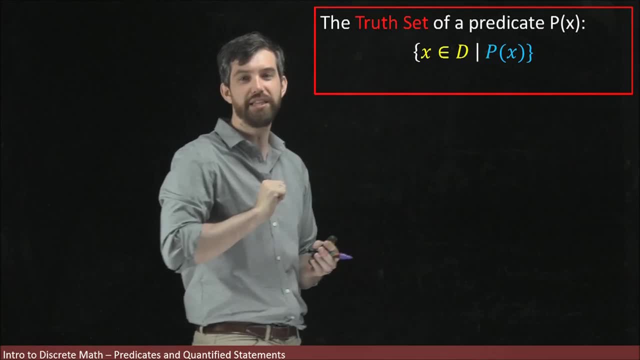 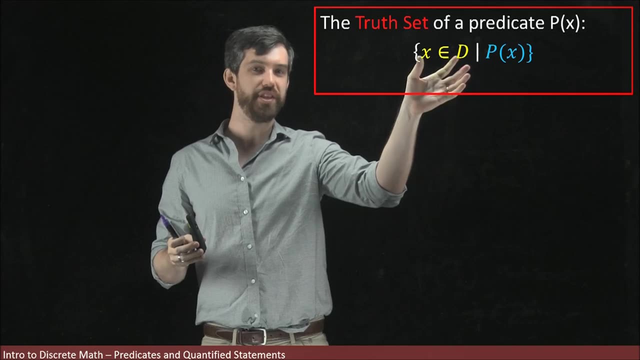 And we've got a bunch of fancy mathematical notation here, so let's try to interpret what that means. This is set builder notation and the first part says the set of all values of x in the domain, so all input values, all the things in the domain. 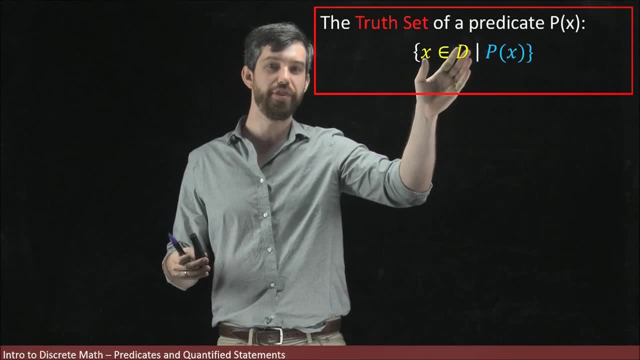 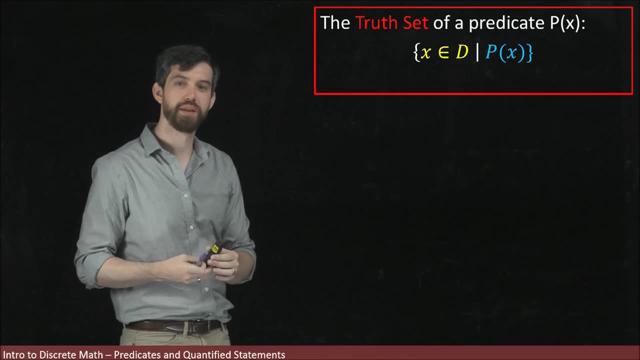 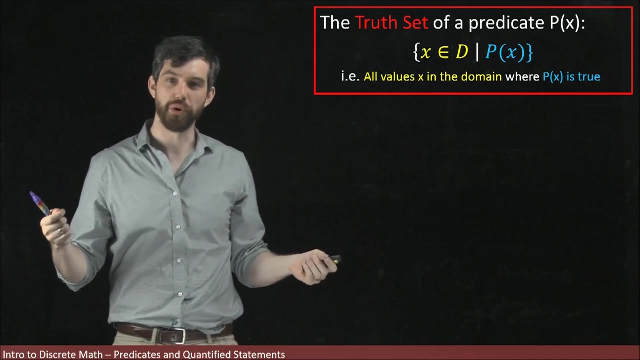 And the vertical line means set such that. so it's all things in the domain such that some property is true, where this property is a predicate. So I can translate this to say: all values of x in the domain where the property is true. That is, to think about the truth set. 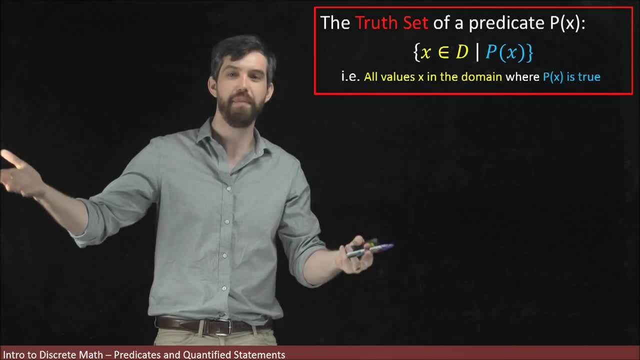 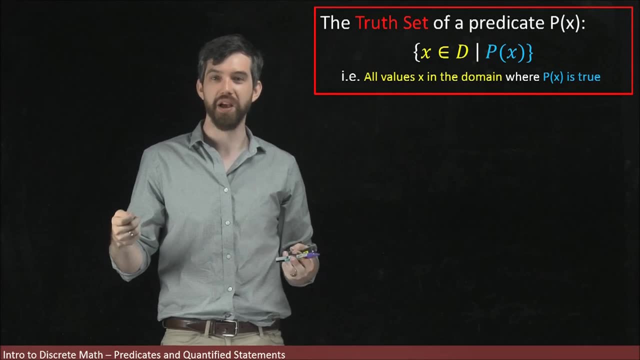 it's just telling me a listing of which of the elements in my domain, which of them make my predicate true. You could also imagine analogously a false set, which would be all the values of the domain where the predicate was false. So let's go back to the example that we had already. 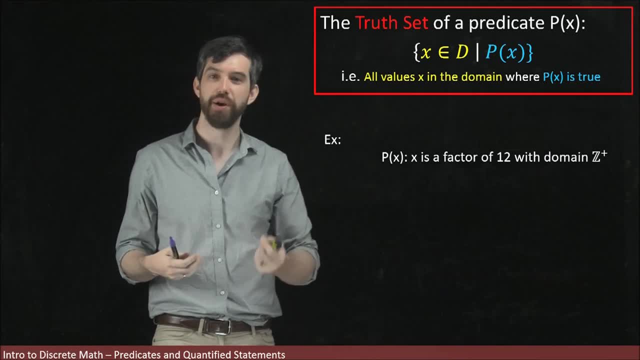 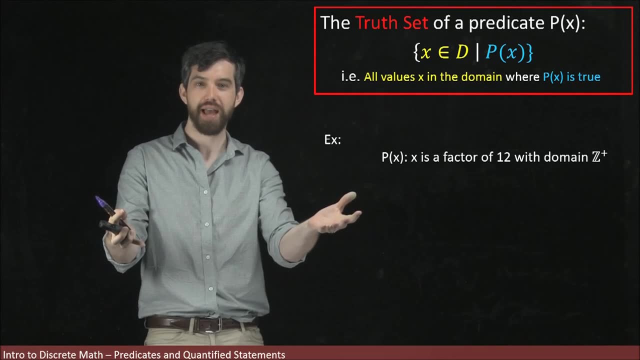 It was this one where x is a factor of 12, with the domain the positive integers. So if I want to write out well, which of the integers have this property, Which of them are factors of 12? I know what all the factors of 12 are going to be. 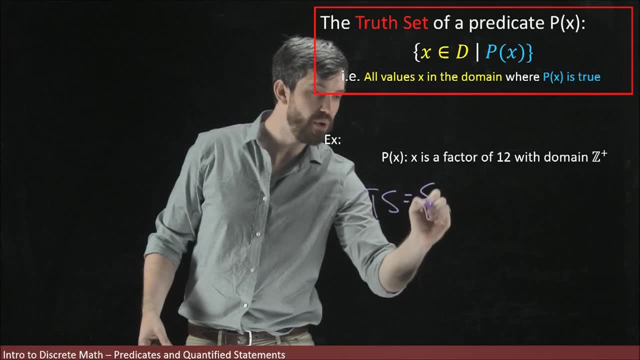 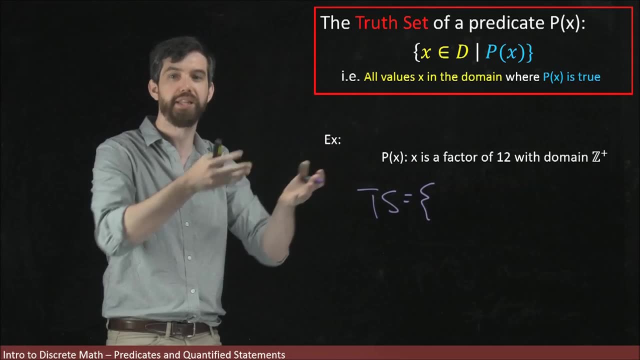 so maybe I'm going to say that my truth set and I'm going to list these not in the set builder notation, I'm going to use set roster and actually explicitly write down what my numbers are going to be. Well, 1 is a factor of 12,. 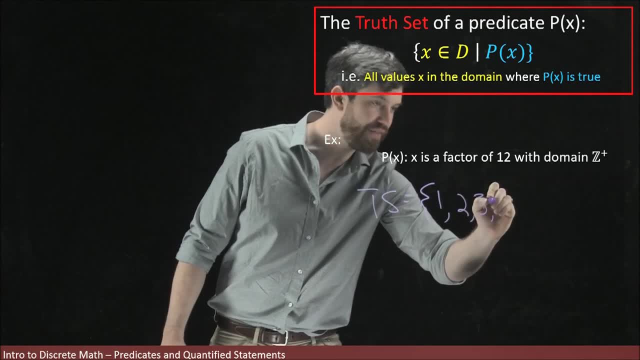 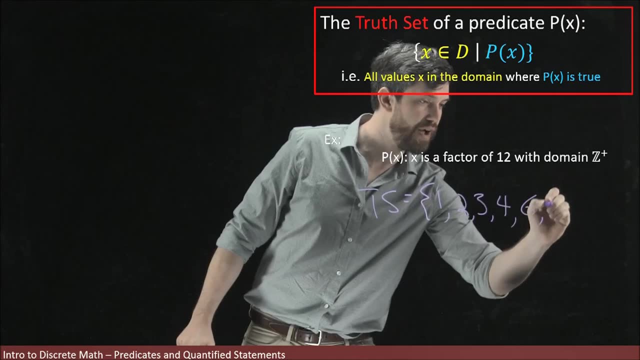 and 2 is a factor of 12, and 3 is a factor of 12, and 4 is a factor of 12,, 5 is not a factor of 12, and then 6 is, and finally 12 is. 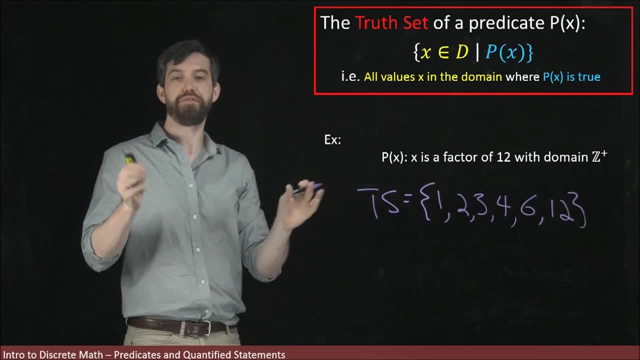 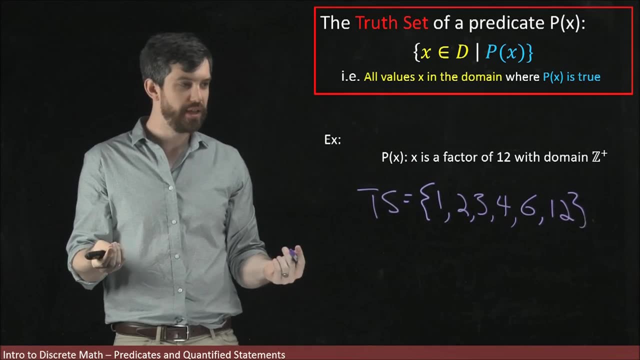 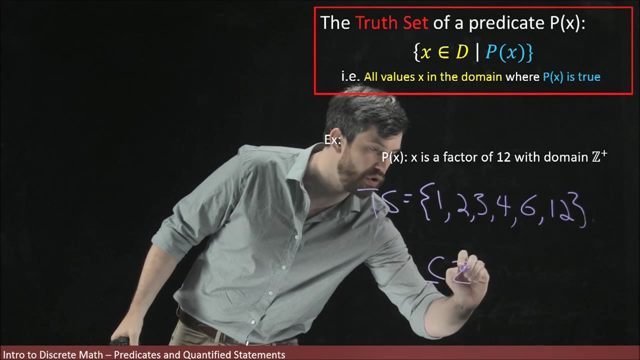 So that's my truth set. Those are all the different factors of 12.. Note that all of the things in this truth set are positive integers. They're not all positive integers, they're just some positive integers. So what I have here is a subset of the domain. or in other words, a subset of the positive integers.